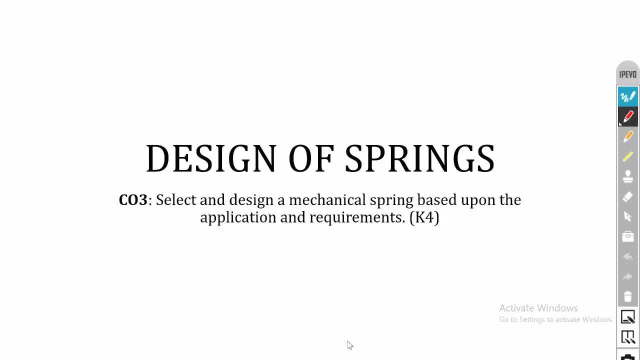 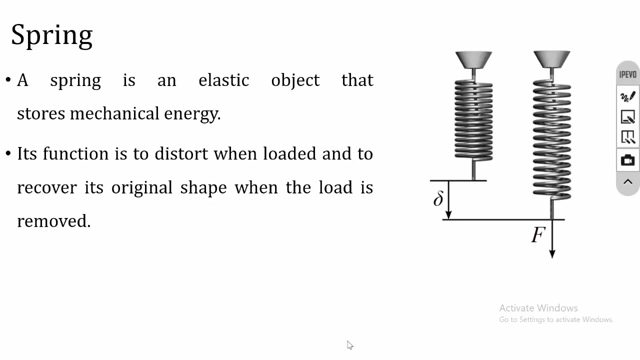 In this lecture I am going to start the third CO, that is, design of springs. So the CO statement is: select and design a mechanical spring based upon the application and requirement, and the CO level is K4.. First, what is meant by spring? So spring is an elastic object that stores 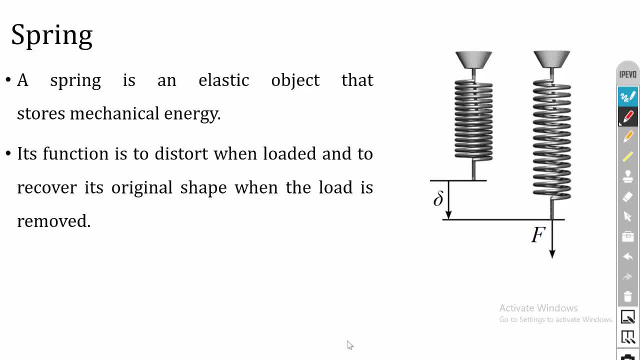 mechanical energy. So the spring absorbs the mechanical energy when it is subjected to external loading and it releases the energy when the external load is removed. So this is the normal state of the spring. When the spring is subjected to a compressive load, then the deflection takes place. So the deflection is named as del. So the spring is an elastic. 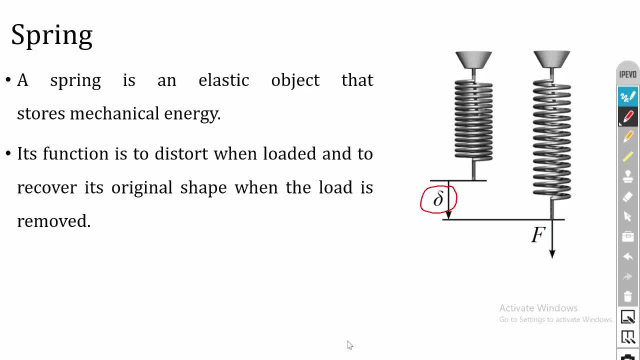 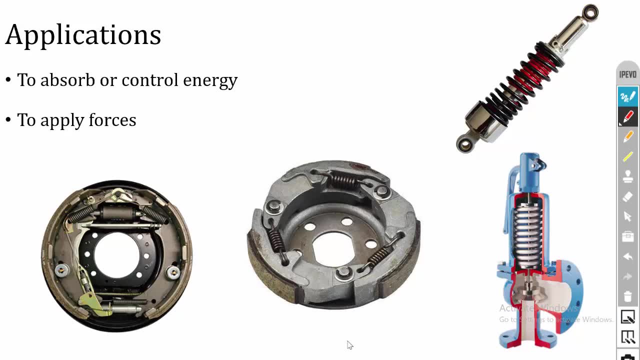 member. That is why, when the load is released, the spring will come back to its position. So the spring is an elastic member. That is why, when the load is released, the spring will come back to its original position. The applications of spring. So, in general, 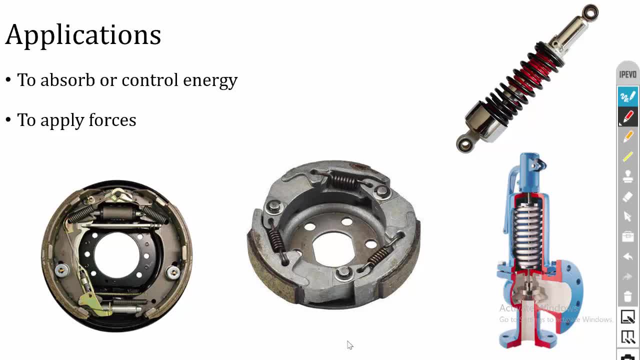 the springs are used in shock absorbers and vibration dampers to absorb the energy. So in shock absorbers, because of the sudden impact, sudden energy is produced, So there the suspension system will absorb the energy produced by the impulse and it will release. 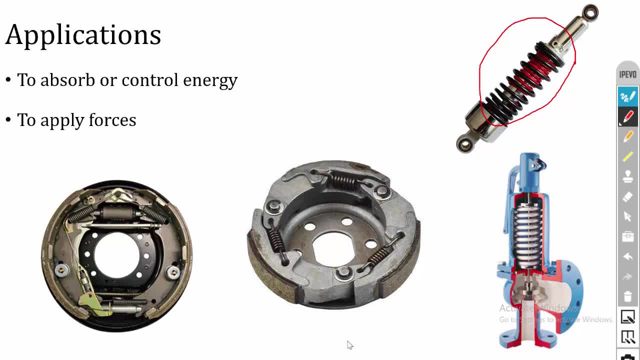 the energy in consecutive cycles. In our two-wheeler and four-wheeler suspension systems, the spring is used to absorb the energy. The second one is to apply forces. So this is a clutch plate. In the clutch plate actually, the clutch is used to engage and disengage the power from the engine to the gearbox. 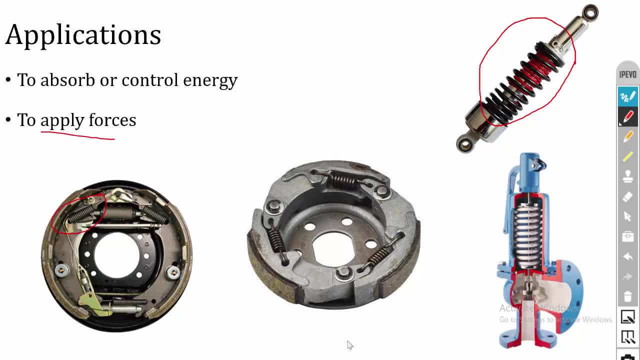 So in the clutch plate you can see that the spring is used to apply the force. That force is applied on the clutch plate And in the case of brake, the force is applied on the clutch plate. In the case of brake, the spring is used to apply the force on the brake shoes And 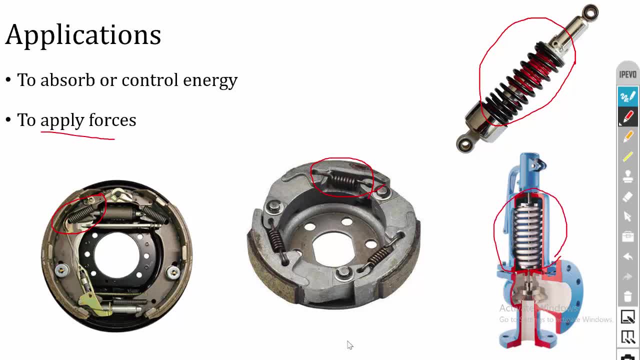 also in some pressure relief valves. So generally the pressure relief valve is used to release the pressure when the inside pressure is above some critical point. So there the spring is used to apply the force on the relief valve. Then in cams, So in cam and follower systems, 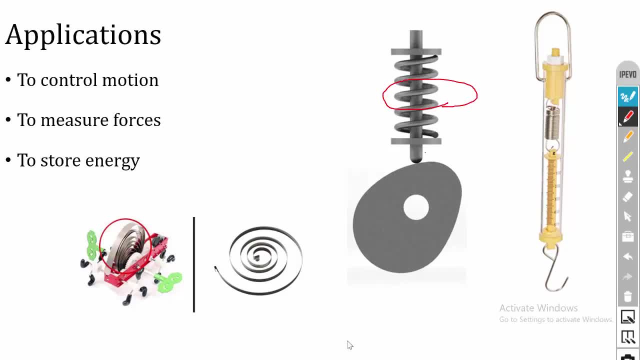 the spring is used to bring the contact between the cam and the follower. So because of the spring only follower is attached to the cam. Then in spring balance the spring is used to measure the weight. And also in watches and in some Thai cars the spring is used. 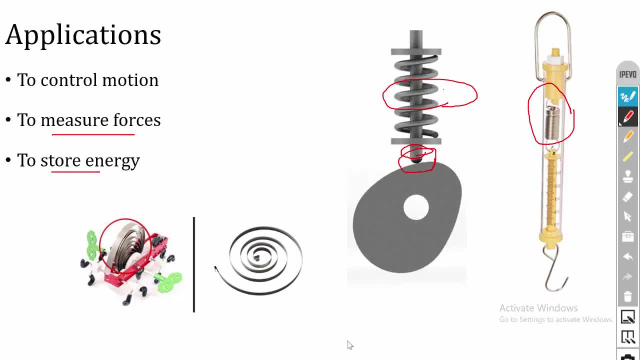 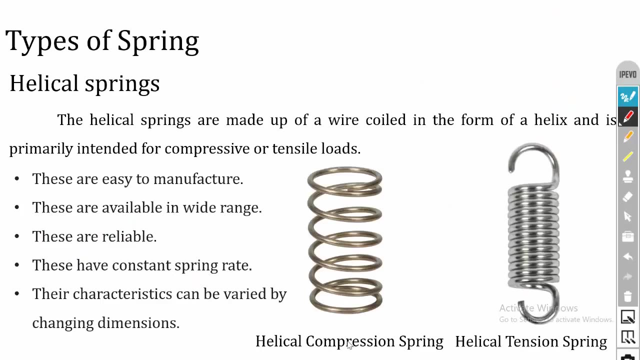 to store the energy, So in Thai cars. so when you apply key then will absorb your energy and when you release the key then the toy car will move because of the energy stored in the spring. So these are all the applications of spring. 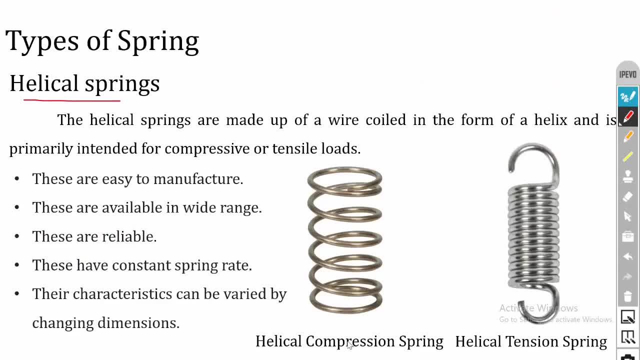 Now the type of spring. So the first and most common used spring is a helical spring. So there are two types of helical springs are there? One is a helical compression spring and another one is a helical tension spring. So the helical compression spring is subjected to compressive loads and in the case of helical 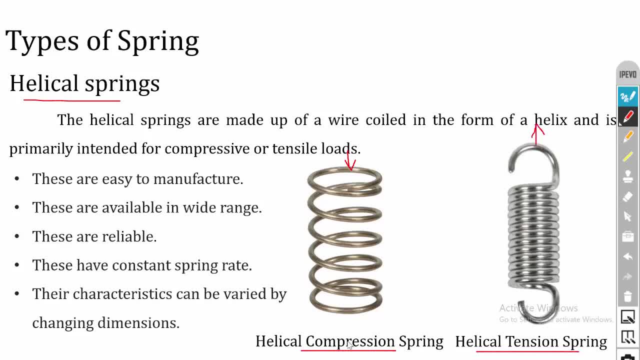 tension spring. the spring can withstand tensile loads. So the advantages of helical spring is these are easy to manufacture, These are available in wide range. Then these springs are of course reliable, Then these have a constant spring rate. Then their characteristics: 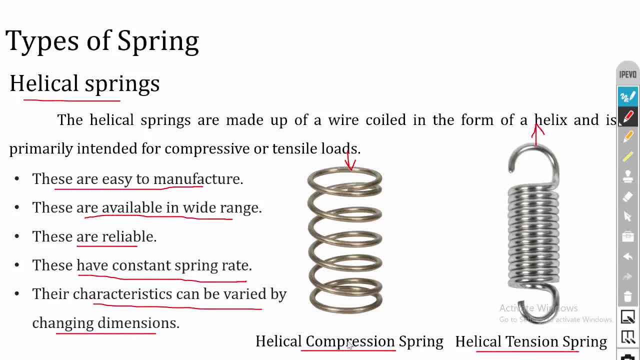 The characteristics can be varied by changing the dimensions. So characteristic means the stiffness of the spring. So this stiffness of the spring can be varied by changing the product dimensions. May be the wire diameter or the coil diameter. So these two factors are mainly affecting the stiffness of the spring. 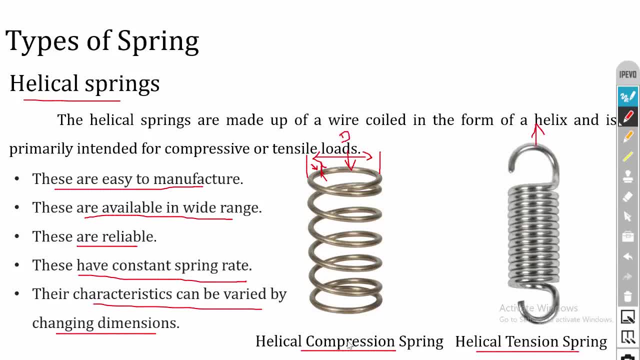 So this is the wire and the small d is wire diameter and capital D is the coil diameter. So these are all the important advantages of helical spring. So those are the main benefits of helical spring. The next one is conical and volute springs. 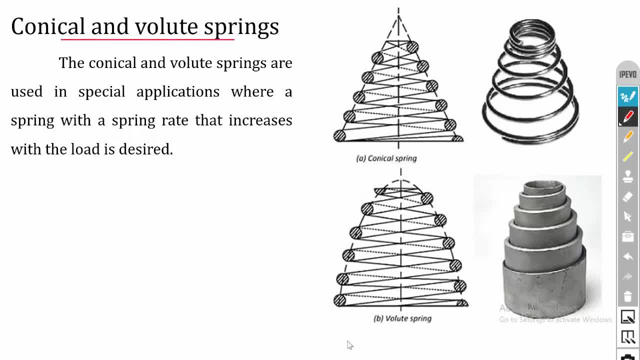 So these springs are only used for some special applications. So these springs differentiate from helical compression and helical tension spring only in the direction, So conical shape and the parabolic shape. So these are all some special springs. Then helical torsion springs. 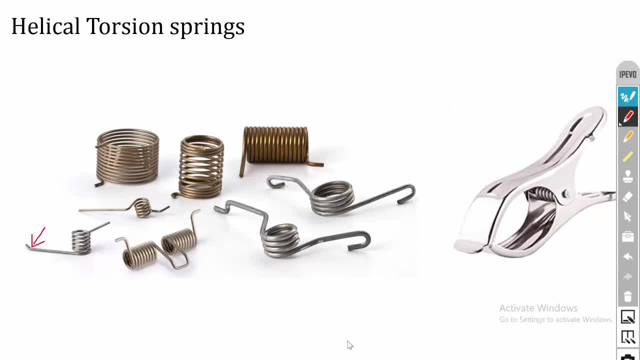 So helical torsion spring will absorb the torsion. So helical torsion springs. We hope you liked this video. torsional loads- okay. so this part is fixed in a board and if you apply a torsional load on the opposite pin then it will absorb the torsional loads, okay. 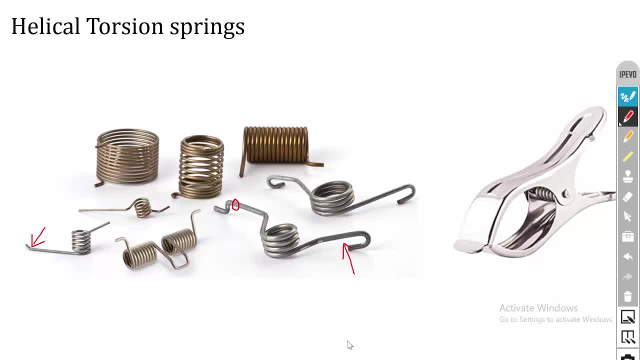 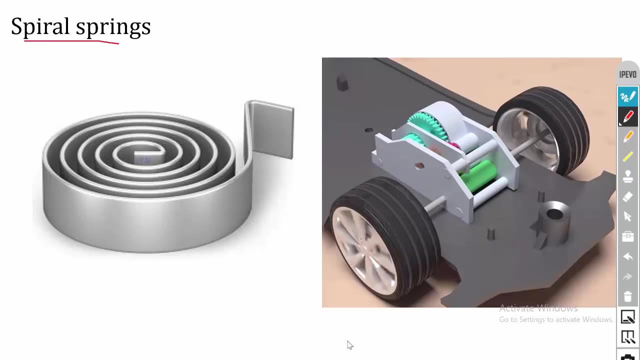 so this springs are used in exam pads, then cloth clips and in your hair clips, okay. so these springs are used to absorb the twisting movement, fine. the next one is spiral springs. so these springs are used in the watch and in the tie cars. so these springs are used to store the energies in tie cars. you might have seen. 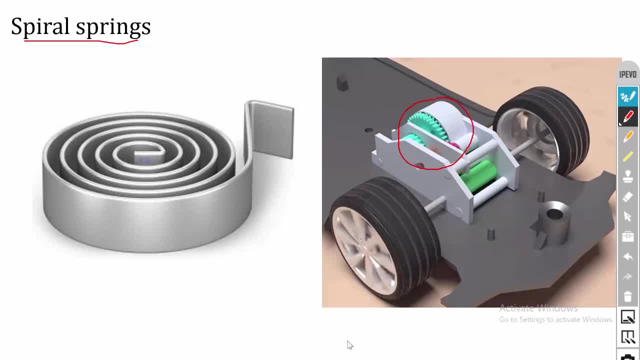 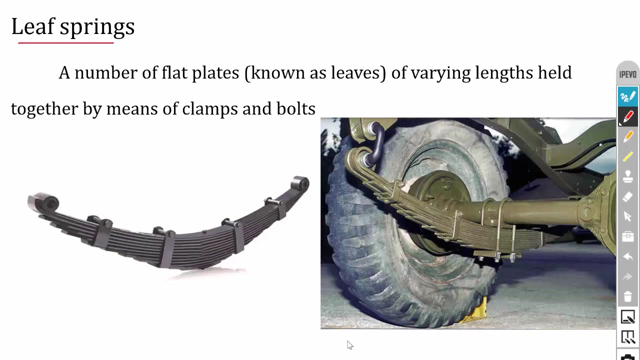 this kind of spiral springs. so this spring is used in tie cars to store the energy. of course, in the generators and in some of the wood cutting machines, this spiral spring is used to store the energy. okay, fine. then the next one is the leaf spring. so it's a very important spring in your four wheeler, okay, so this? 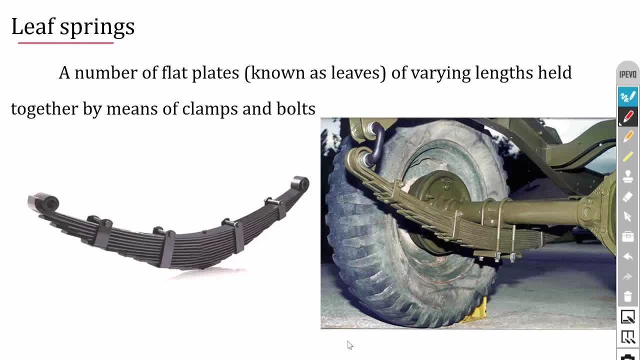 spring is used in our four wheel suspension system to resist high amount of force. so here a varying length of leaves held together by means of bolts and clamps to apply the load. so these are all different leaves with varying lengths and these all held together by some clamps and bolts to apply the load. 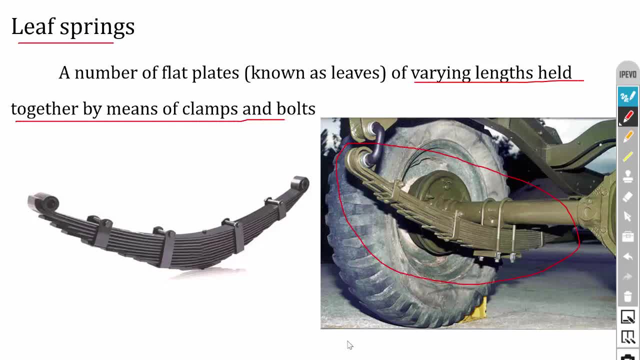 okay, so this spring is used in our four wheel suspension system to resist high amount of force. so these springs you can see in your buses and your trucks, so these springs are used to carry high amount of load and this will not give perfect cushioning effect, just like your helical compression and helical tension. 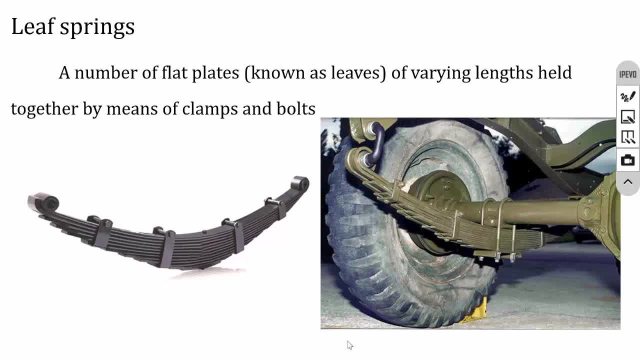 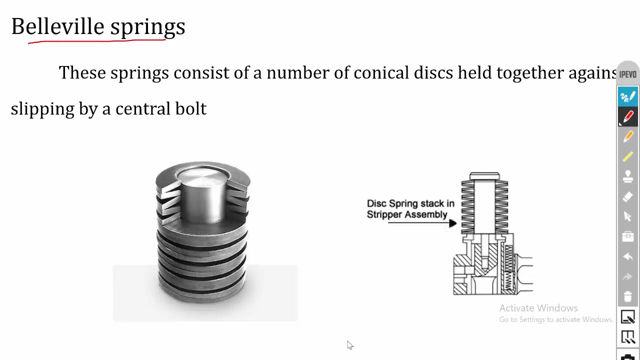 spring. that is why in heavy load applications in your lorries and buses they are using leaf spring, and in our two wheelers and in some of the four wheeler cars they are using helical compression spring to get some good suspension effect. the next one is belly wheel spring. so these springs are formed. 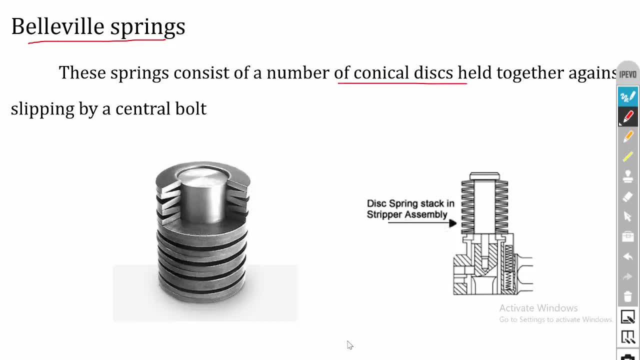 by combining the conical discs. okay, so you can see that many conical discs are combined to form a belly wheel springs. okay, so these springs are used in some of the valve assemblies. okay, so, to absorb the vibrations of the valve. okay, fine, so now the design of helical spring. so we will start with the helical spring. 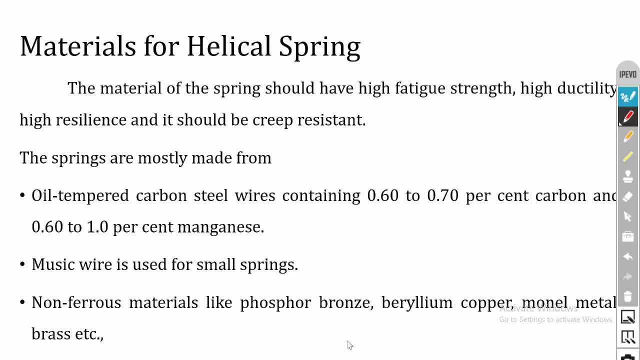 the helical compression spring. so the helical spring is made of oil, tempered carbon steel containing 0.6 to 0.7 percent carbon and 0.6 to 1 percent of manganese. then for small springs, the music wire is used, and in some of the 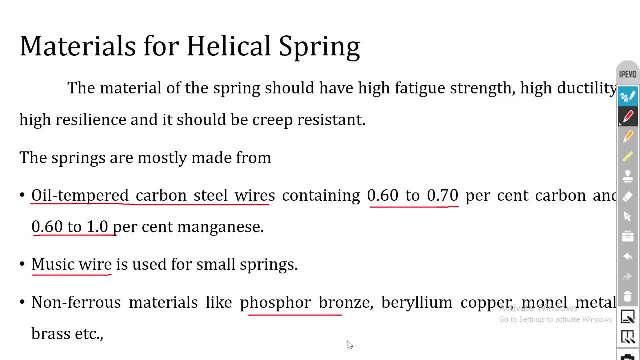 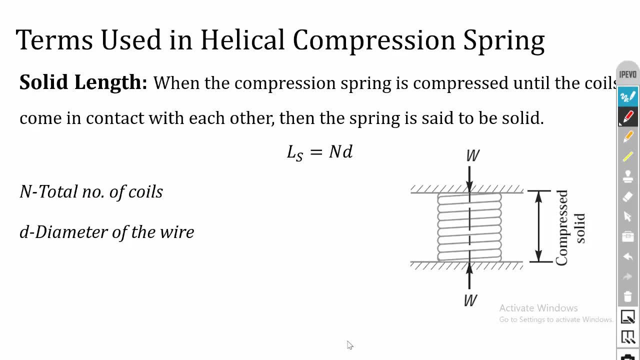 applications. the non-ferrous materials like prosper, bronze, beryllium, copper and monol metal or brass is used for some of the spring manufacturing applications. so the terminology is used in helical compression spring. so the first one is solid length. so you can see the image. so this spring is fully compressed, so there, 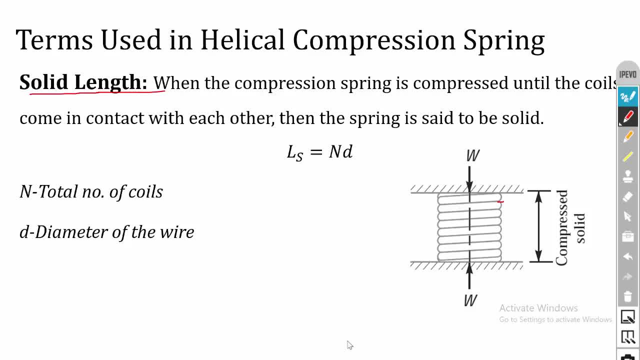 is no gap between the two adjacent wires. so in that state the length is called as solid length. so when the spring is fully compressed, then the length of the spring is called as solid length. and the equation for solid length is n into d. so here d is the wire diameter. so the diameter of a single wire times the number. 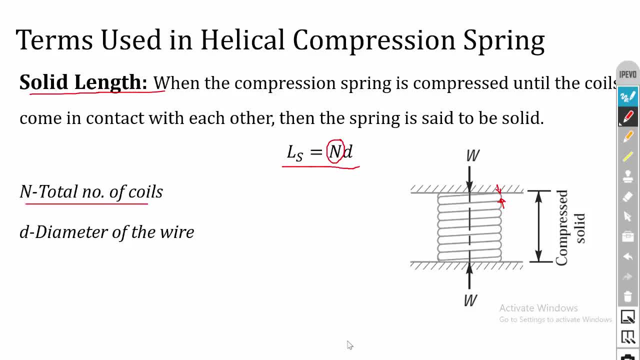 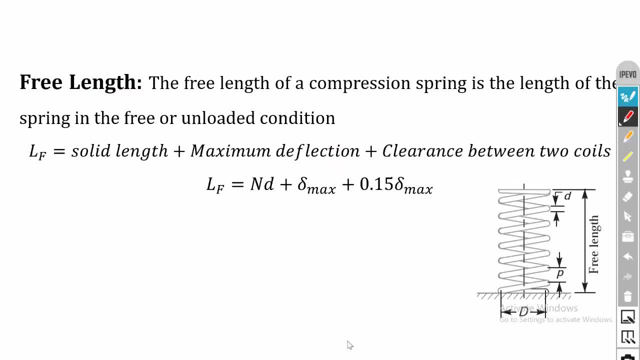 of turns. okay, fine, so n is the total number of coils and d is the diameter of wire. so this is the solid length. then if the spring is free from compression, then your spring will be like this: there will be some gap between the two adjacent wires, so that in that state 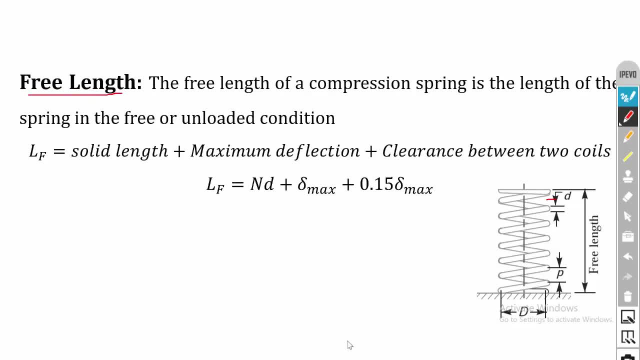 the length is called as free length. okay, so there is no load is applied. that is why it is called as free length, and the free length can be calculated by. lf is equal to solid length plus maximum deflection, then plus clearance between the two coils. okay, so lf is equal. 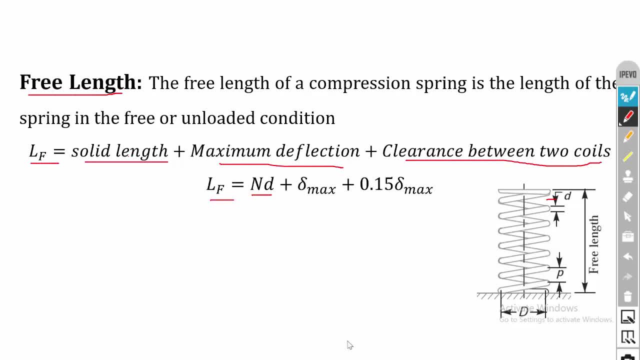 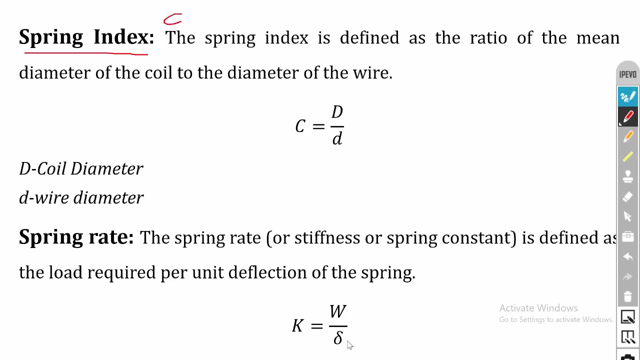 to solid length is n into d, so that we have calculated earlier. then the maximum deflection is del max. Further, the clearance between the two coils is 0.15 into del max. okay, so this is the clearance between two coils. so this is the free length lf. the next one is spring index, that is c, so the spring index. 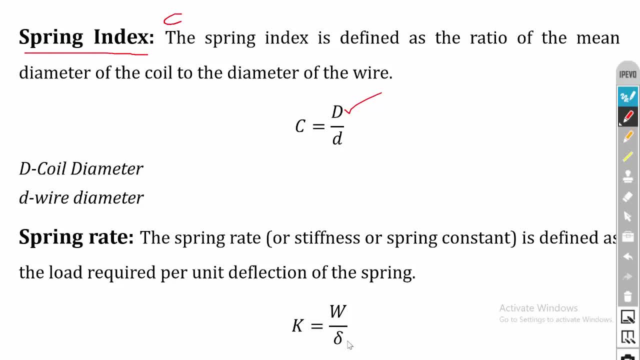 is the ratio between wire diameter, and I mean the coil diameter and the wire diameter. so if this is your spring, then the overall diameter is coil diameter, that is capital d, And the diameter of the individual wire is small d, that is the wire diameter. okay, so 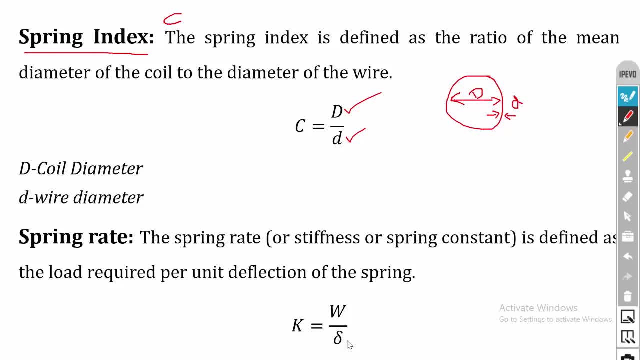 spring index is the ratio between coil diameter and the wire diameter. so if in the problem, if the spring index value is not given, you can assume a spring index value of 5, because in most of the springs they will consider the spring index value as 5. okay, so if it, 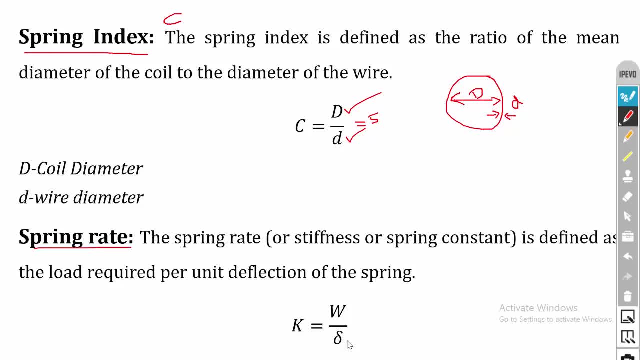 is not given, then you can assume 5, then the next one is spring rate or otherwise. sometimes it is called as spring rate. We know that stiffness is load by deflection. so k is equal to w divided by del. so here I have considered the load as w and the deflection as del. so this k will be very useful to identify. 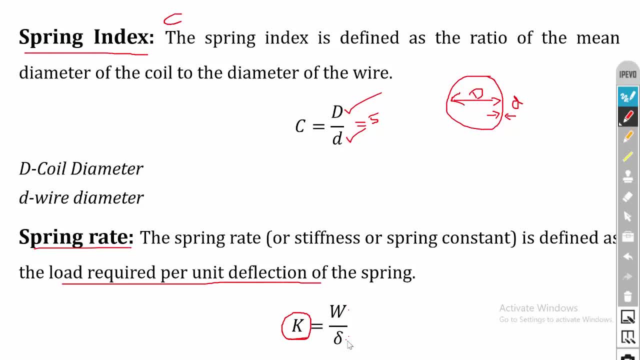 the characteristic of the spring. because if you go into the dynamic side, in the vibration side, the springs are mainly used to absorb the energy. so there they will calculate the natural frequency by using the equation root of k by m. So this m is the mass of the system and this k is the stiffness of the spring. so this k. 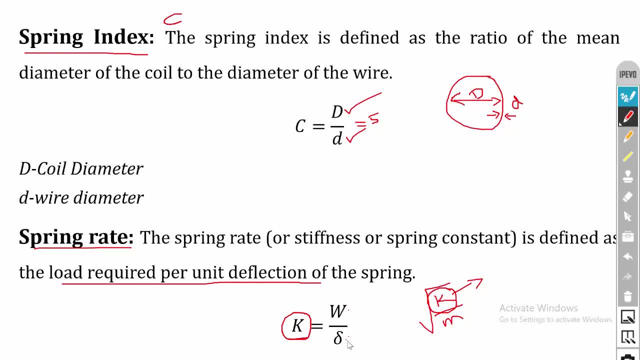 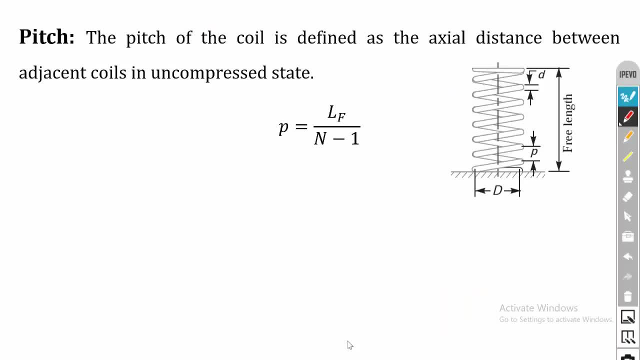 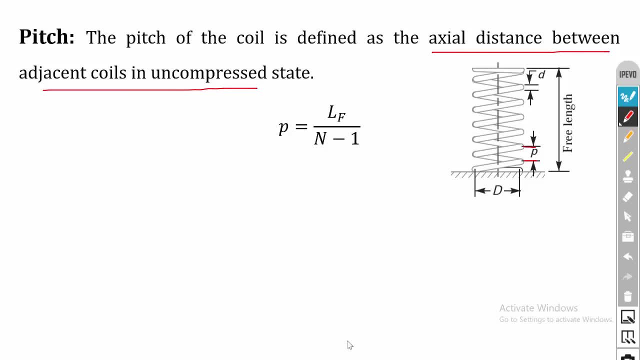 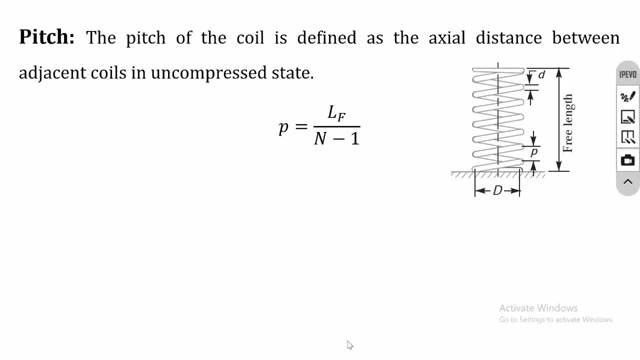 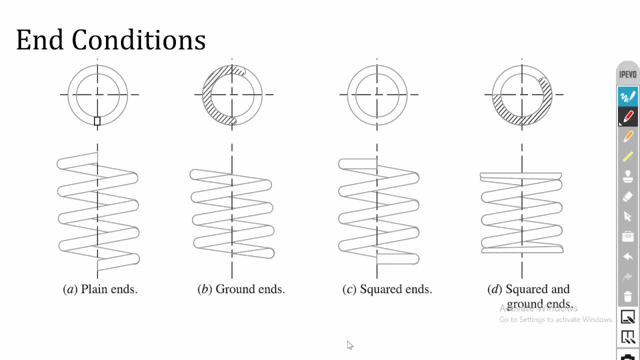 So this is the equation for pitch. So these terms are used in the design of helical compression spring and helical tension spring. Now the end conditions. So actually, if you manufacture a spring, The end conditions will be like this. So the ends will be like this. 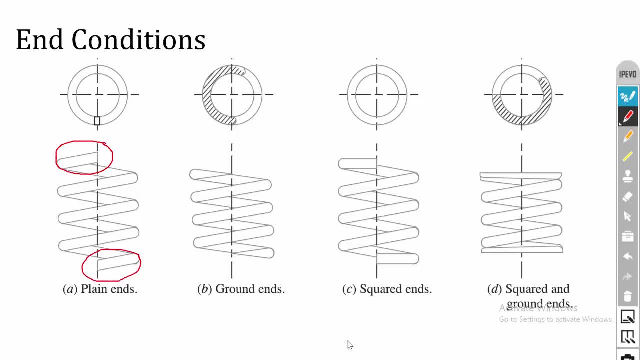 So there is some projection is there. So this is called as plane end Suppose. if you want to carry any load in some cases then you can cut the additional projection here. So you can cut the additional projection of the spring. You can see that. 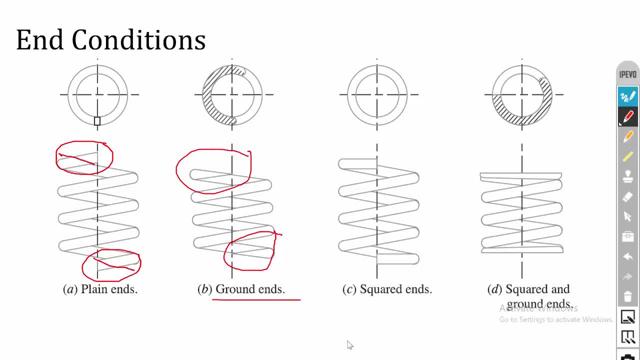 So these are called as ground ends. In some cases they may bend the additional projection. You can see that: Like this, So they have bended. like this, So this is called as square ends. In most of the cases the ends are bended and they are grounded. 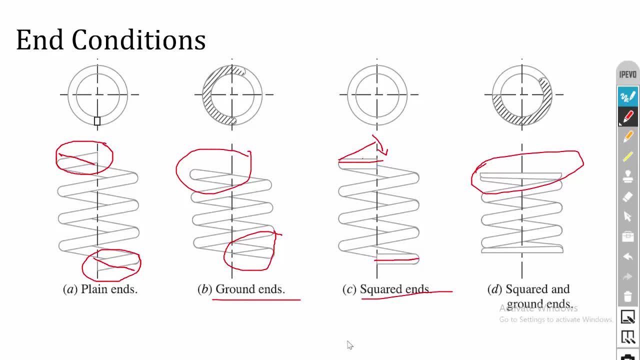 So initially it is bended and the remaining portion is grounded, So this is called as squared and grounded. So in most of the cases to carry heavy amount of loads the helical compression spring is squared and grounded. So this is very important. This condition is most used in load carrying capacity applications. 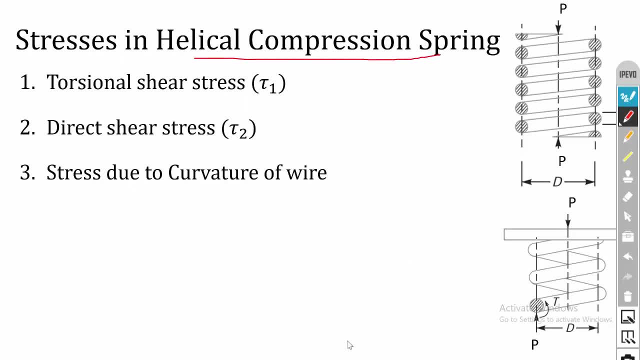 Now the stresses in helical compression spring. So before going to the design procedure We must understand what all the types of stresses are acting in helical compression spring. So the first one is torsional shear stress. So consider a helical compression spring of coil diameter D and wire diameter M. So the 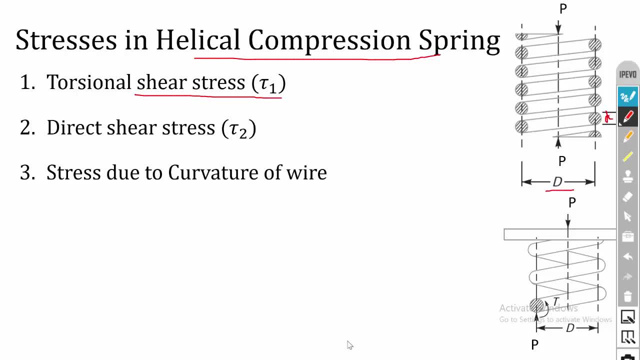 stress in helical compression spring is equal to the pressure acting in the helical compression spring, a load P is acting. So when the load P is acting, then this wires are subjected to some twisting moment. You can see that. So when the load is acting, the wires are subjected to some twisting moment. 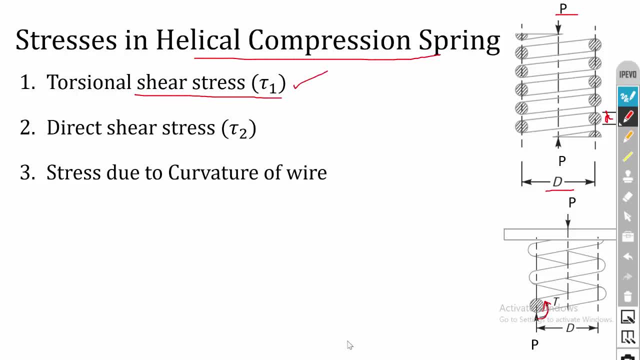 So because of the twisting moment, the torsional shear stress is developed on the wires. So that is the first stress, and the second stress is when the load is applied. then the spring is directly subjected to some shear stress. So that is the direct shear stress that is towed to. 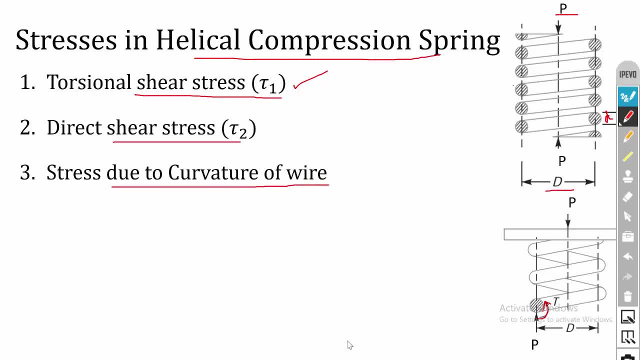 Then because of the curvature. so if you see the spring the outside is subjected to some elongation and the inside is subjected to some compression. So that is because of the curvature effect, and because of this curvature some additional amount of stresses are developed in the spring. 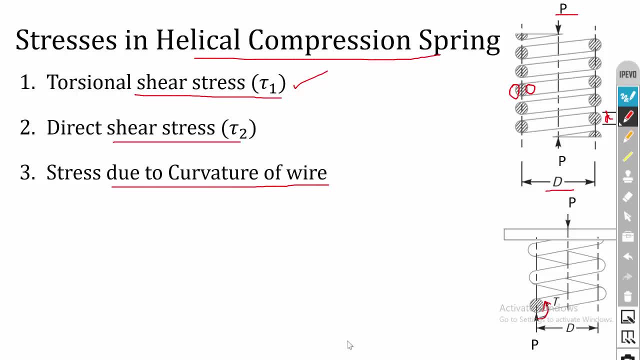 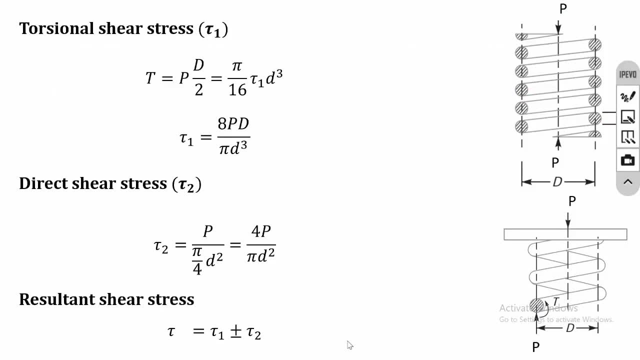 So that is the third one. So now, if you do, If you want to design a spring, first we have to calculate the three stresses are acting on the spring. So first we will calculate the torsional shear stress. So consider the torque acting on the spring as T. 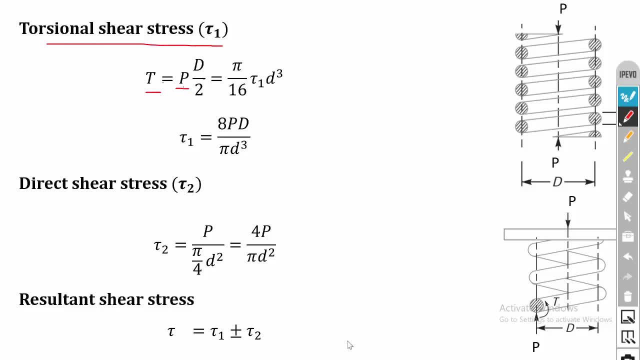 So T is equal to load into radius. So the load is P and the radius is d by 2.. And further we know that the torsion equation is pi by 16. tow into d cube for circular cross section. Now you can see that the wire cross section is a circular one. 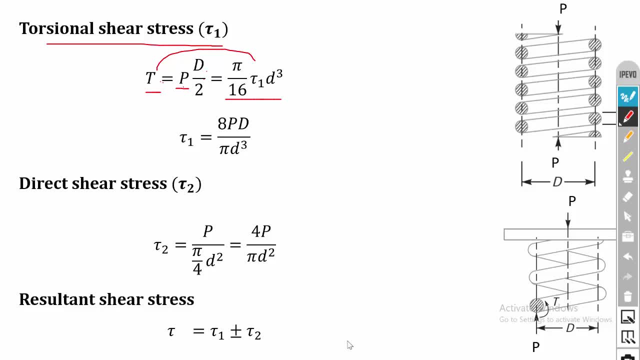 So further. you equate this two, Then you will get tow. 1 is equal to 8 pd divided by pi d cube. So here P is the applied load, d is the coil diameter and d is the wire diameter. So this is the torsional shear stress. 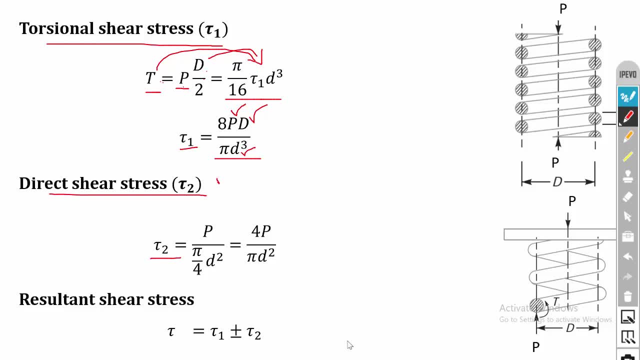 Then the direct shear stress. we know that the equation for direct shear stress tow is equal to P divided by A. So the load is P and the cross section is pi by 4 d square, since it is circular cross section. So further bring the 4: it is 4 P divided by pi d square. So here it is subjected. 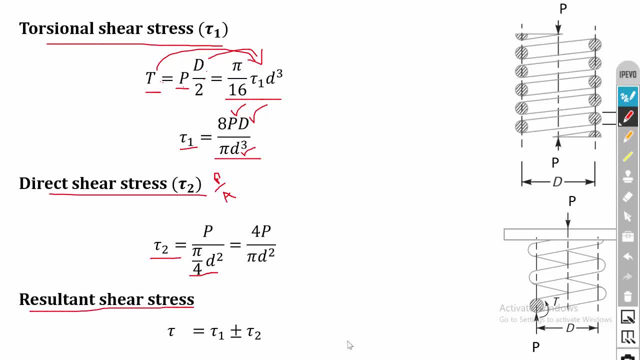 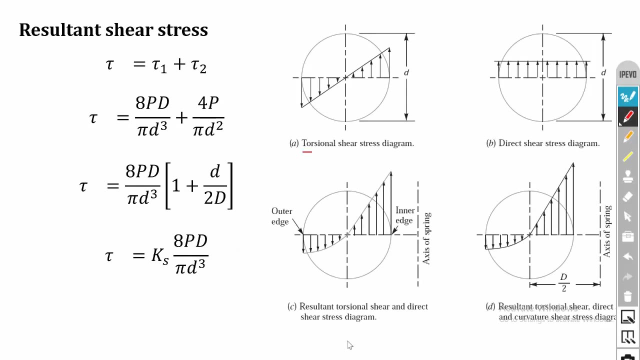 to both shear stress to find the resultant shear stress. then tau is equal to tau 1 plus or minus tau 2.. So now we have to select whether we should go for addition or we should go for subtraction. So for that this images will be helpful. So this is the shear stress drawing. 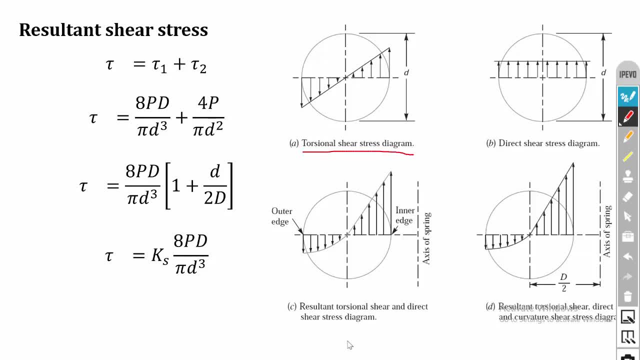 for torsional shear diagram. So the inside is subjected to a force moving towards upward and the outside is subjected to moving downwards. So this is torsional. We know that the torsional is acting in the rotating direction. That is why we are getting two opposite forces. 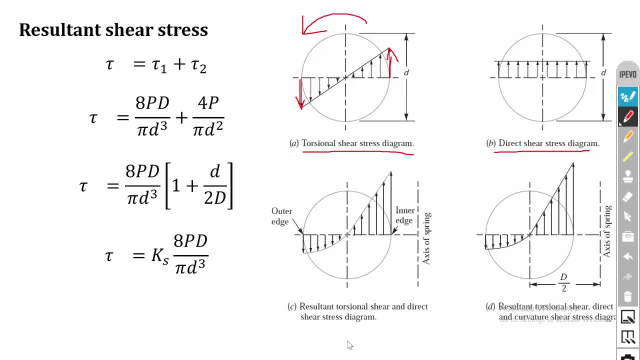 Then the second one is direct shear stress. So here the torsional is acting in the rotating direction. So here we are getting two opposite forces. All the forces are acting towards upward. So when we add these two force, then what will happen is we will get a maximum stress value. When you subtract these two forces, then what? 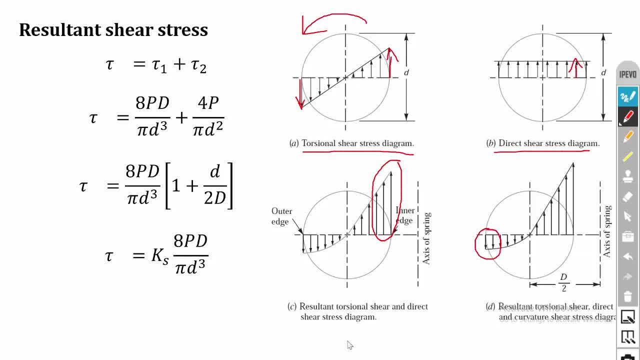 will happen is the stress value will be minimum. We know that while designing any component, always we should select the higher stress so that the system will not undergo any failure. So we have to select the inside part, So we have to consider the addition That is tau. 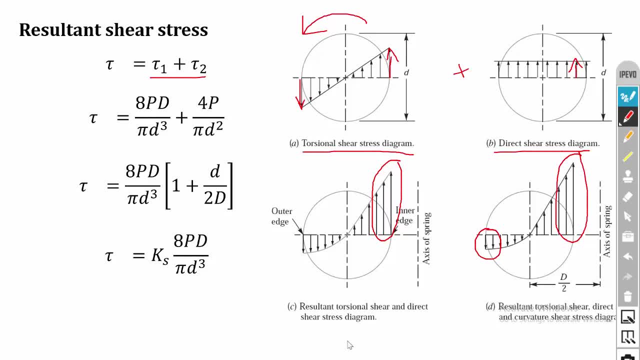 1 plus tau 2.. So now you can substitute the value of tau1 and tau2, and here I have taken the 8pd divided by pi d cube outside, so I will get 1 plus. here there is no d component, so I have multiplied. 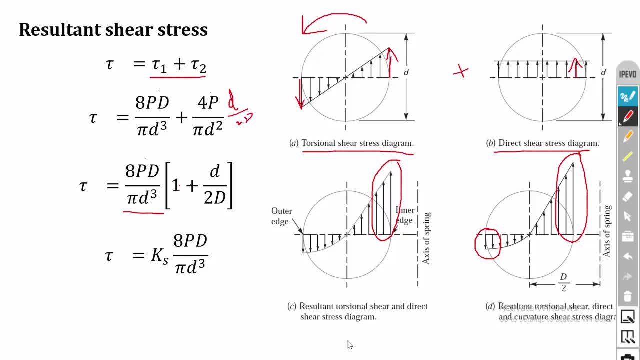 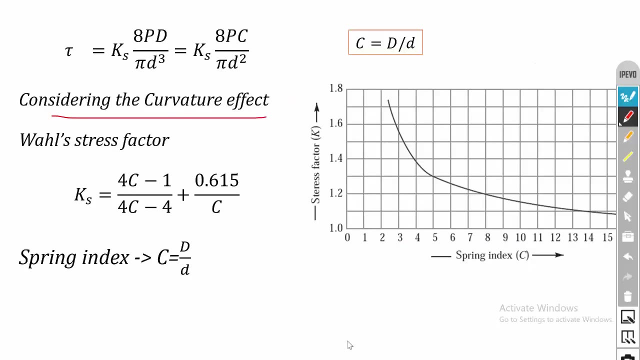 d divided by 2d. so I will get 1 plus d divided by 2d. here I have replaced this 1 plus d divided by 2d by a tam ks, so I will tell you what is ks later Further to consider the effect of curvature. so initially I have told you 3 stresses that 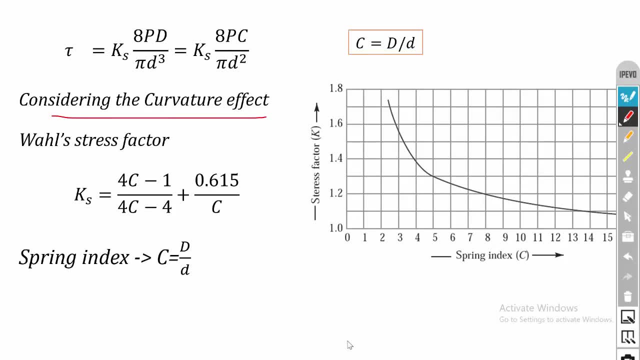 is direct stress, torsional stress and stress because of the curvature. so previously we have considered 2 stresses and for considering the curvature effect we are going to consider the wales stress concentration factor, that is ks. so here I have replaced the ks, that is 1 plus d divided by 2d. 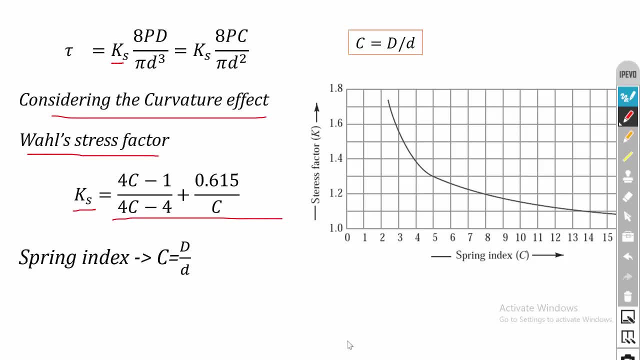 So this is the factor for considering the curvature effect, that is curvature stress. so this chart will be useful to find the curvature. so the x axis is spring index, that is c, that is capital D divided by small d. so if you know the x axis then you can automatically 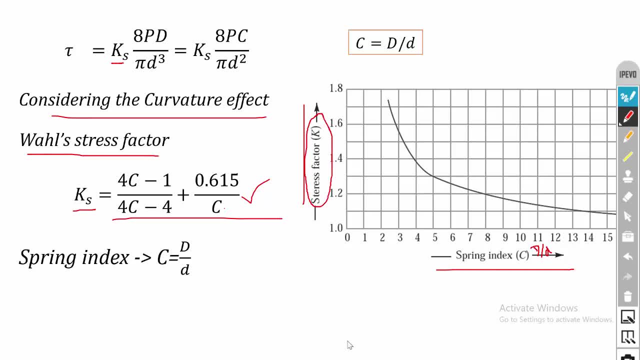 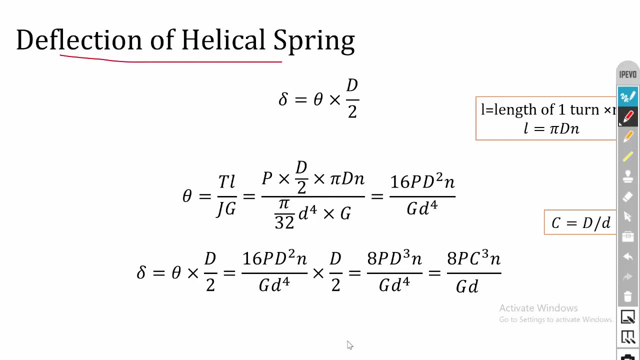 select the y axis, that is stress factor. Otherwise you can use this equation to find the wales stress equation. So all these data are available in the data book. You can see that. So before that we will calculate the deflection on the helical spring. 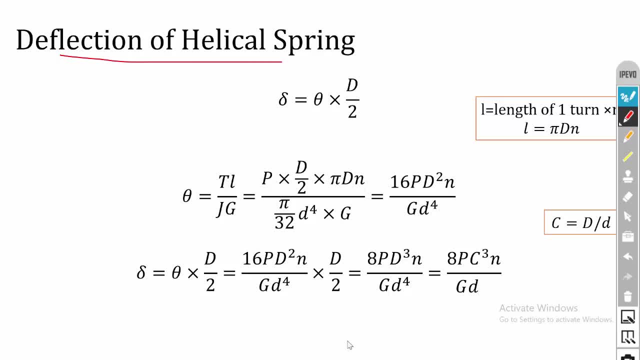 So the deflection del is equal to d theta into d divided by 2. so theta is the angle of twist into the radius. So for a circular system deflection is equal to angle of twist radius. so here the radius is d by 2. so further we know that the data is equal. 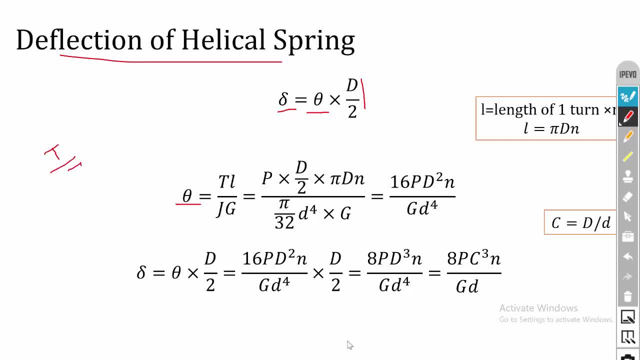 to. we know the torsion equation is: T by J is equal to G, data by L. so here I have kept the data in the left side and bring the remaining term to the right side. that is TJ divided by J, G. so here T is torque. we have already calculated the. 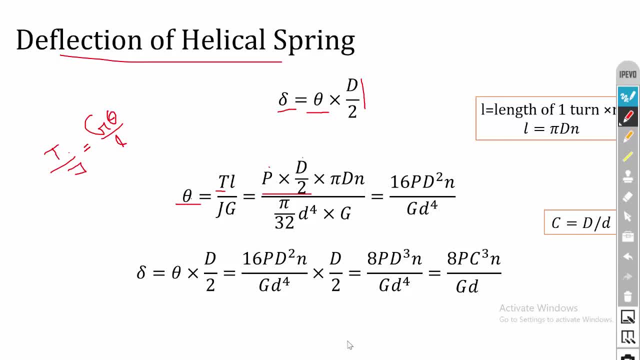 torque value earlier. that is, load into radius, it is P into d by 2, and L is the length of the spring. ok, so here we should be very careful that the length of one spring is pi into D. circumference of the spring is the length of one turn. 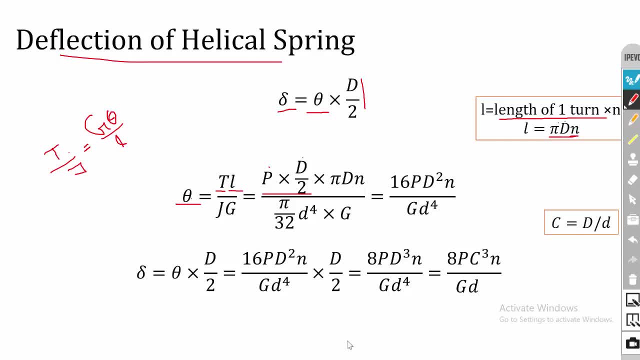 that is pi into D. so if you want to calculate the length of overall spring, then it is pi into D, into the number of coils. so it is pi D n. so in the place of L you can substitute pi D n. then we know that for circular section J is equal to pi by 32. D power 4, substitute the value. 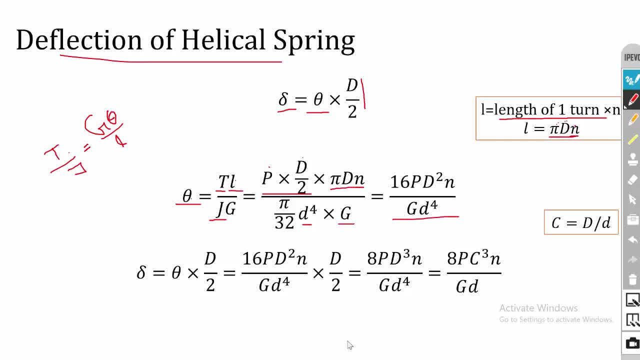 of G and calculate data. so further, after calculating data, you can substitute the data in the first equation, you can simplify the terms. so finally you will get 8 P, D cube N, divided by G, D power 4. so here P is the load, D is the wire. I. 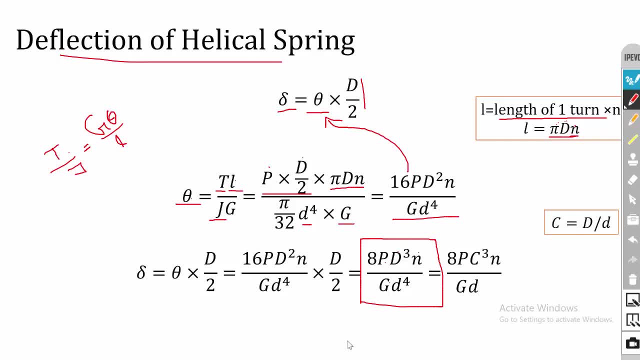 mean coil diameter, N is the number of turns, G is the modulus of rigidity of the spring and small d is the wire diameter. further, we can replace this capital D by small d by C, because we know that C is equal to capital D by small d. so we can use C cube, so that here you will get. 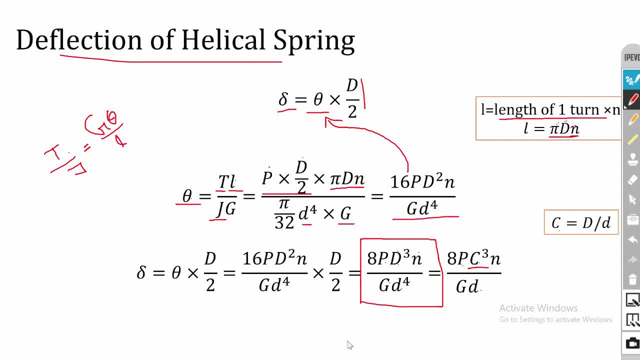 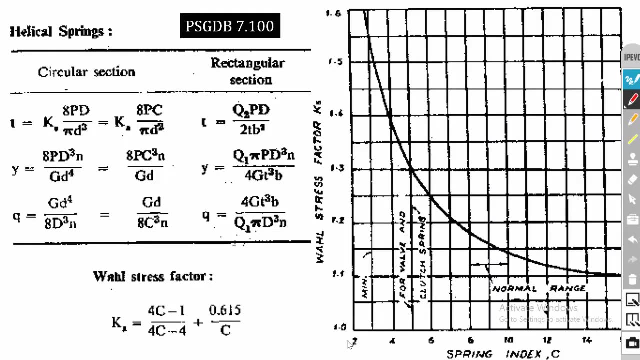 only D, so it is 8 P C cube, because D cube, D cube will get C cube N divided by G D. so these two equations are very important, that is, the stress equation and the equation for deflection. and all these equations are available in data book, page number 7.100, so you don't need to memorize anything, okay? so here,